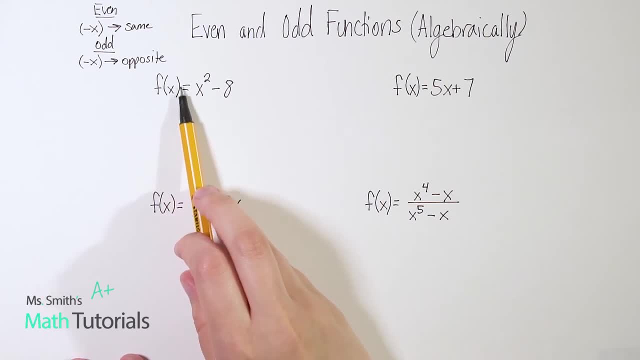 this. remember, this is a function. This means f of x. It's just a fancy way of saying y x squared minus eight. So I'm going to plug in negative x and see what happens when I simplify. So I'm going to put in negative x squared minus eight. Now, negative x squared. 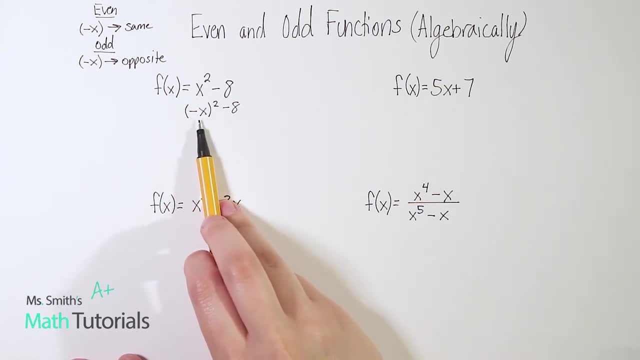 so that's negative x times negative x, and hopefully you remember that a negative times a negative is a positive. Parentheses here are so important. So this is actually going to end up being positive x squared when you simplify that minus eight. Now notice once. 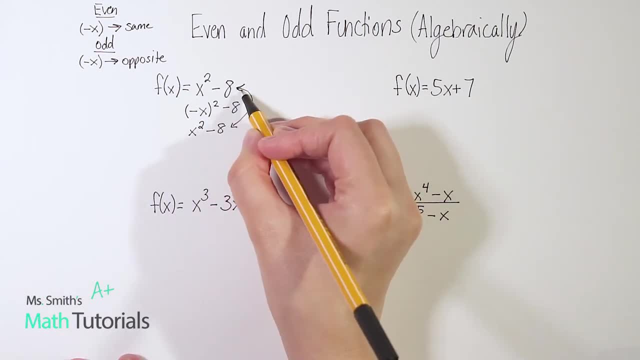 we simplified. compare that to what we started with and you'll see they're the exact same right, This one's positive, this one's positive, That one's negative, this one's negative. So, because they're the same, this is even. 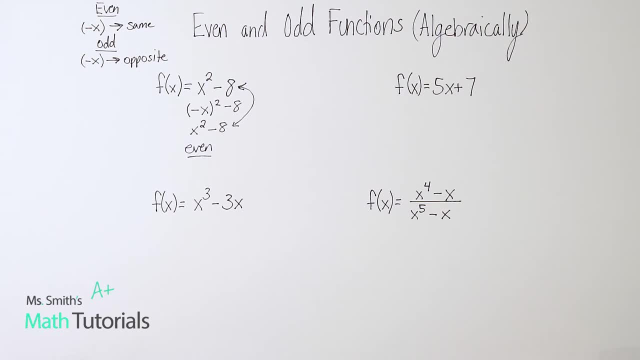 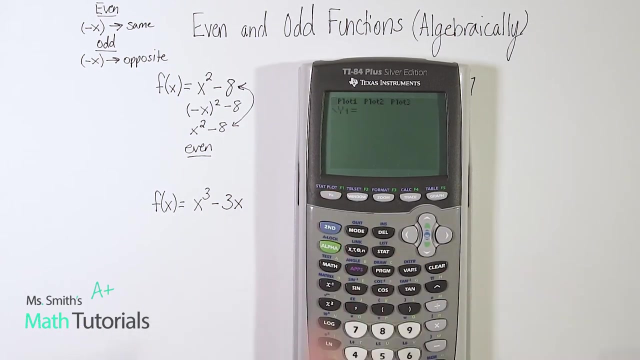 Okay, Now let's check that on the calculator because we want to be sure, And I think I always find this is a great way to catch any possible mistakes that you've made. So the way I'm going to check this is I'm going to go to my y equals and I'm going to type in: this is y equals. 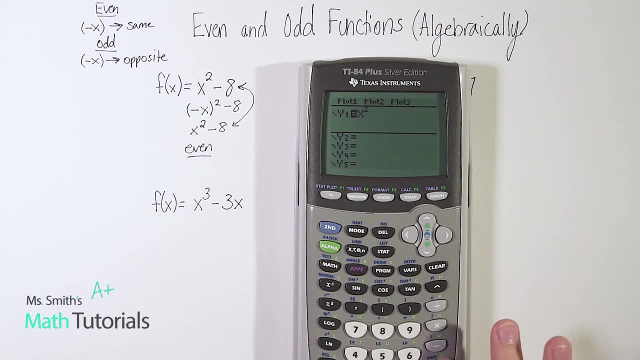 so I'm going to type in x squared, x squared minus eight, And I'm going to graph it. Let's just look at it. Okay Now, especially if you watched the last video on how to identify even and odd functions graphically, you'll 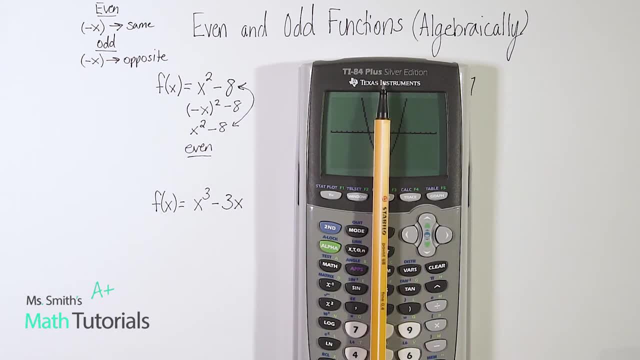 remember that if it is mirrored across the y-axis, that means it's even So. that just confirms with me that I did do this right, okay, and with you as the viewer. So that's a great tool. So we'll use that each time just to double check our answers. 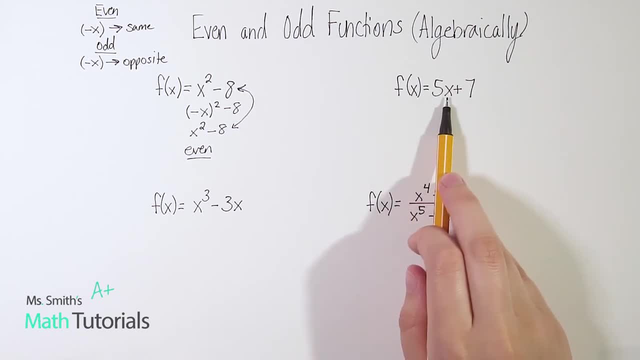 Let's try this one. So remember: instead of x we're going to plug in negative x and see what happens. All right. so five times negative x plus seven, All right. well, five times negative x is going to be negative. five x plus seven comes down. Now let's compare. 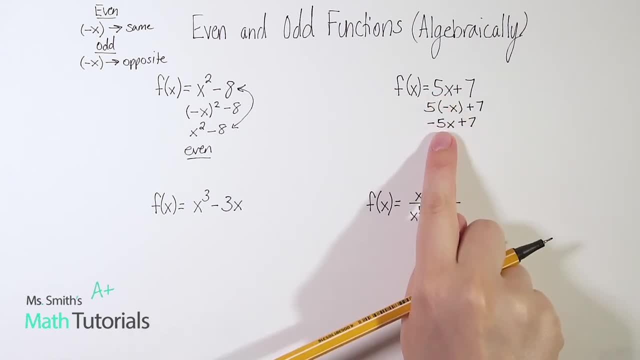 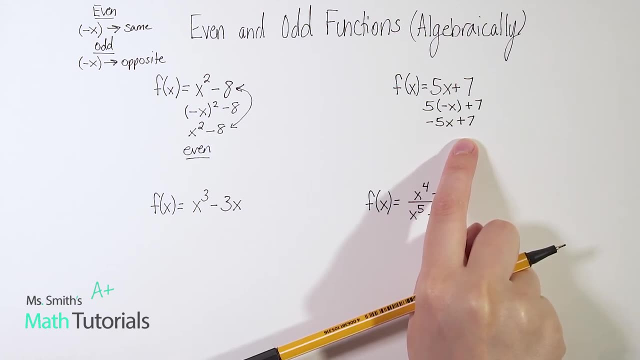 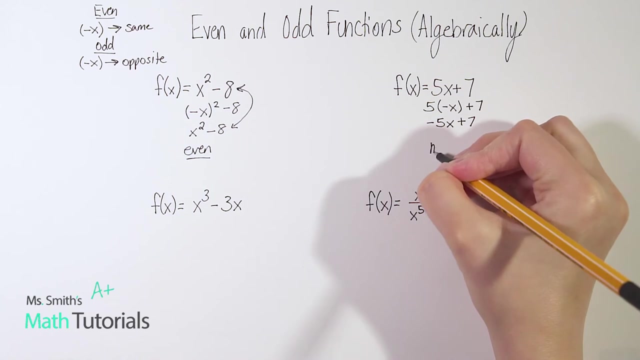 that to what we had to start with The five flip sign. The seven did not. So this is not the same and it's also not opposite. So even though this one is opposite, every single sign would have to be opposite. So this one's neither. 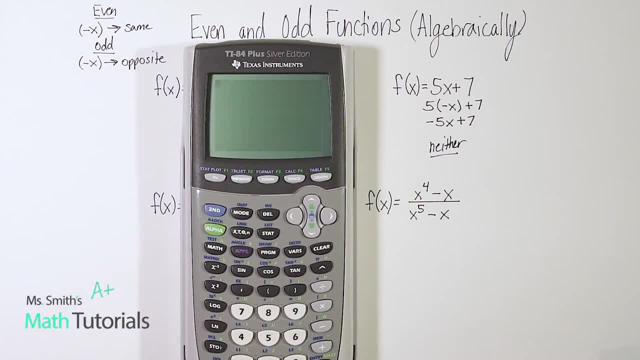 And let's check it using our calculator, just to be sure. So we go to our y equals. You'll see I had what I previously put in there. Clear that out. Five x plus seven. I'm just putting in what I originally had. and let's look. 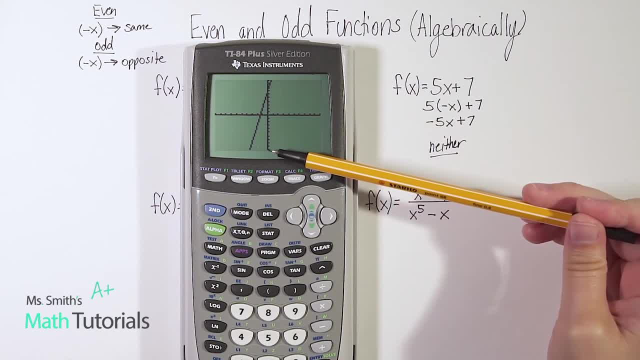 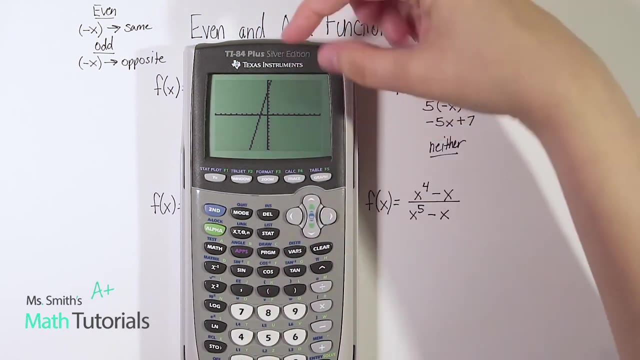 So I can tell this is not mirrored across the y-axis, because it would have to be perfectly the same on one side and the other and it's not. It also if I were to flip this upside down, which I'm actually going to do, because I can easily do that with my calculator notice. 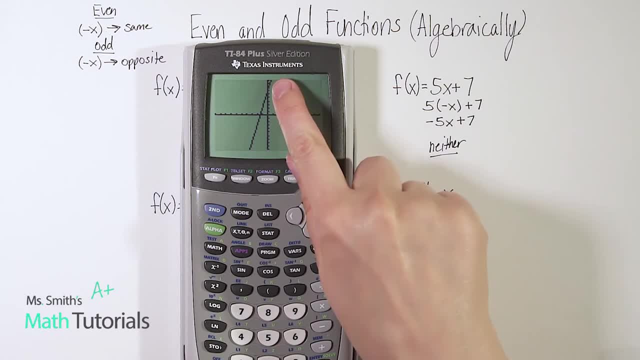 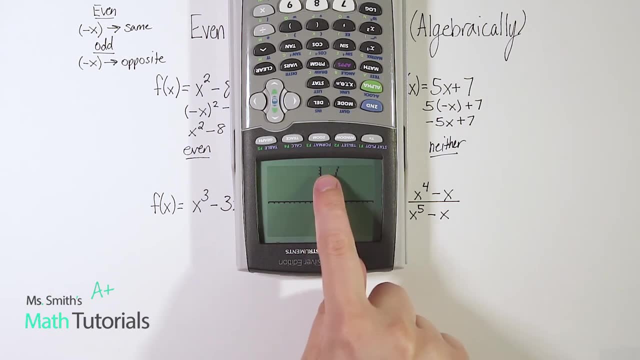 how I have a wide space at the bottom and a little space up top. Well, if I were to flip this Now, I've got wide space up top, little space at the bottom, And if this was truly odd, it would be the exact same. It would be the same proportion. So this just confirms that. 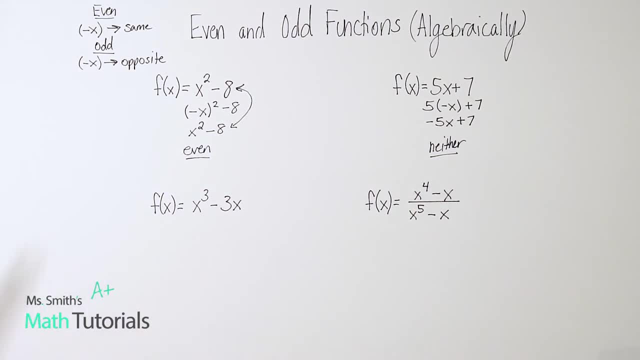 this is neither, and I can keep moving. All right for the next one. So I'm going to plug in negative x every time I see an x, So I have to do it not only here, but here as well. Minus three times negative x, And 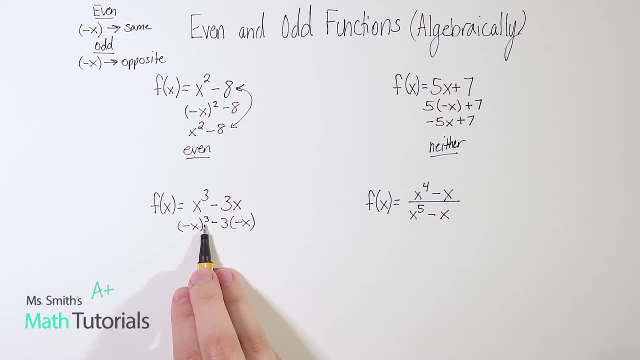 we're going to simplify Now: negative x cubed. So that's negative x times negative, x times negative x, And that one actually does leave me with negative x cubed. Now negative three times negative x. that's going to leave me with a positive three x. So compare that to: 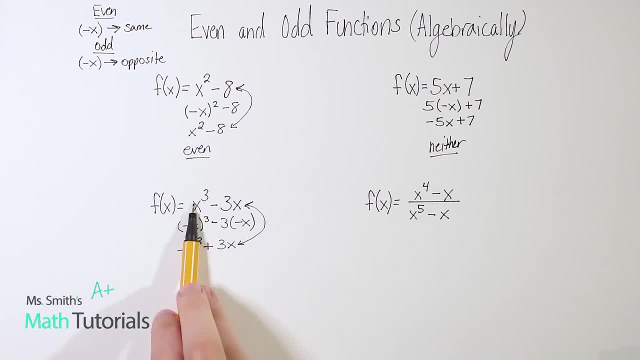 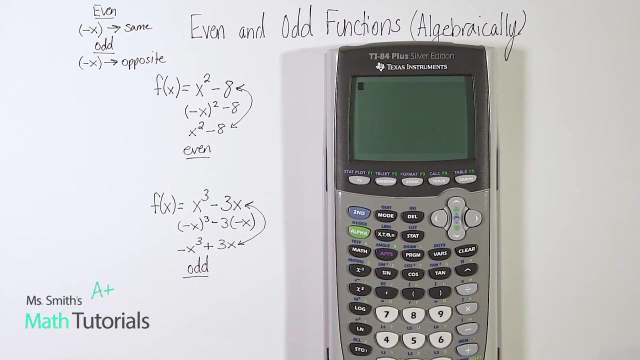 what we had at the beginning And you'll see that the x flip sign and the negative three x flip sign. So that means remember if it was opposite. that means this is odd. Let's just confirm using the calculator. So we go to our y equals. clear out what was previously in there: X cubed minus three x. 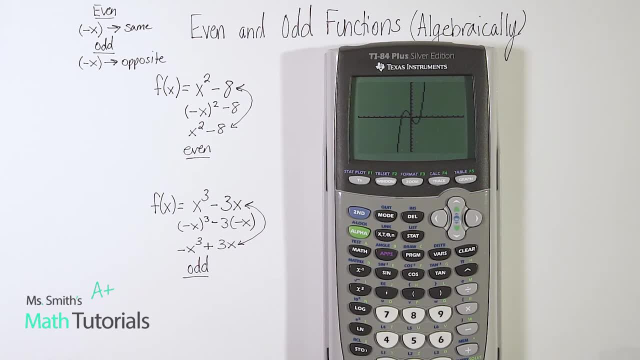 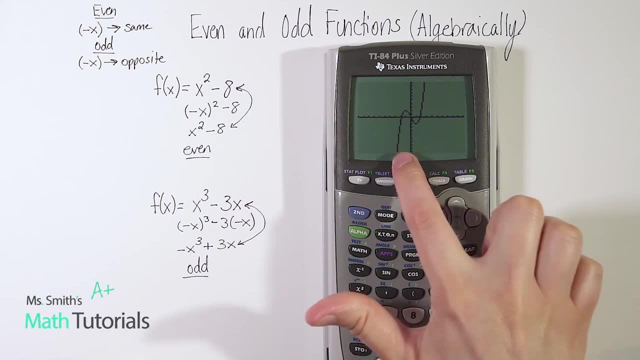 Let's just see what it looks like. Okay, now notice, I can't reflect it, So it's definitely not even. But notice, here I got kind of a wide space on the bottom, kind of wide space up top. a little little dip there. 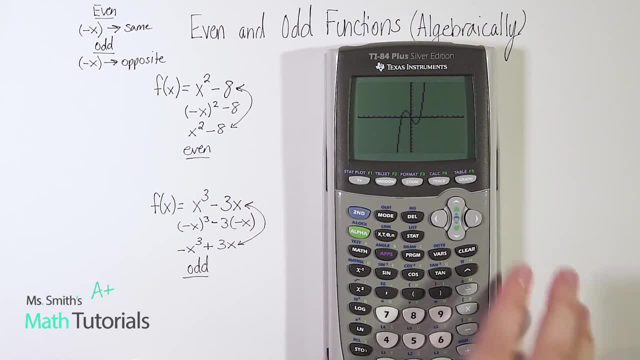 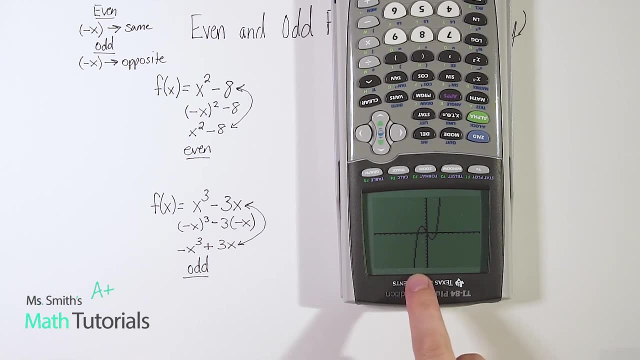 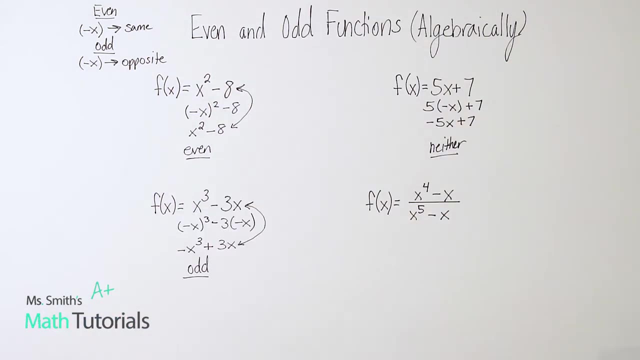 You definitely want to take note of those characteristics so that when you flip it and you compare, you see it's the exact same. Space there, space there, Bump down, bump down, Bump up- it's the exact same. So that just confirms that this is, in fact, odd. 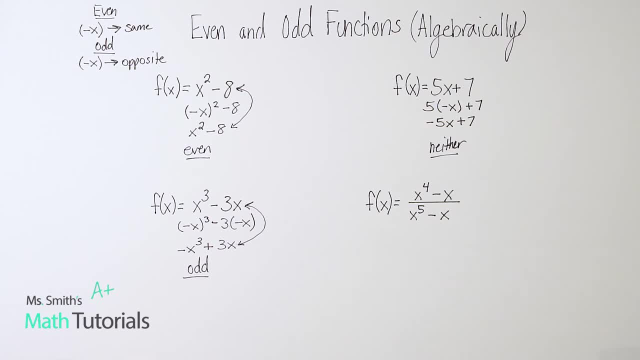 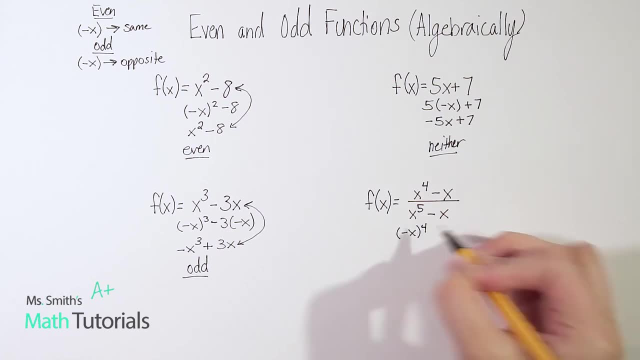 Let's try this one Now. this one looks weird, right, because it's got that fraction, But we still treat it the same way. We're going to, instead of writing x, we're going to write negative x to the fourth minus. 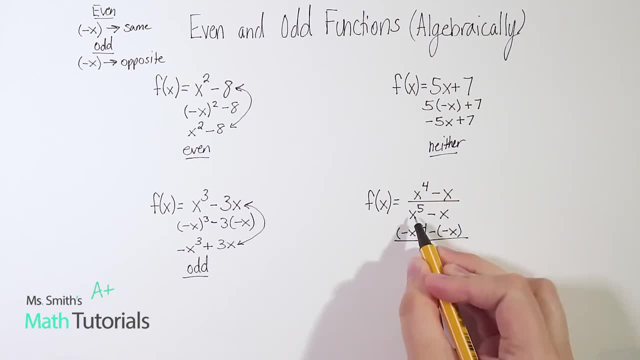 negative x. And then on the bottom, we're going to put negative x to the fifth minus negative x. We're going to write negative x to the fourth plus negative x, plus negative x, minus negative x. There we go. So I said x to the next 1.. 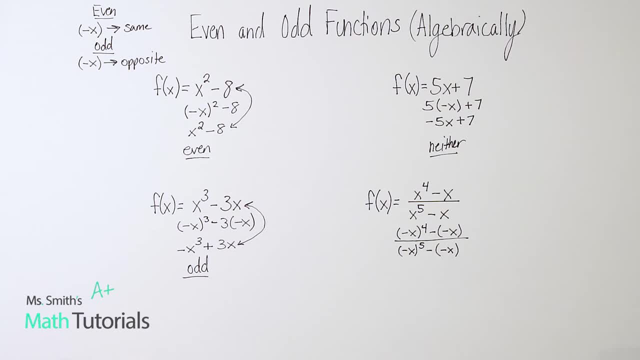 Negative x is negative for x, squared Negative x and negative x to the fourth. So careful with numbers, because we're going again, we're going to take big numbers. So, for example, negative x to the fifth minus negative x. 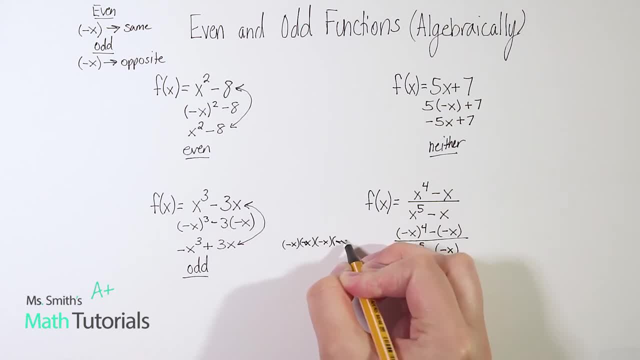 So I won't get too lucky here. I haven't done the first. Yes, I'll must, but you didn't catch it. Okay, there we go. Okay, well, that's positive x, right, x squared. excuse me, positive x squared, and then x squared times. 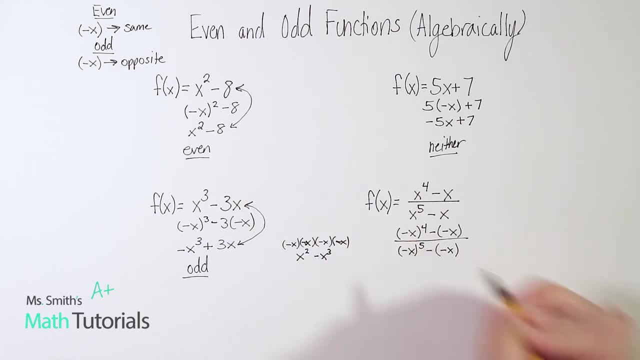 negative x- well, that's going to be negative x cubed negative x times negative x- well, that's going to be positive x to the fourth. okay, so this reduces to positive x to the fourth. another way of thinking about it is, if this is an even number, this is going to reduce to a positive, so you 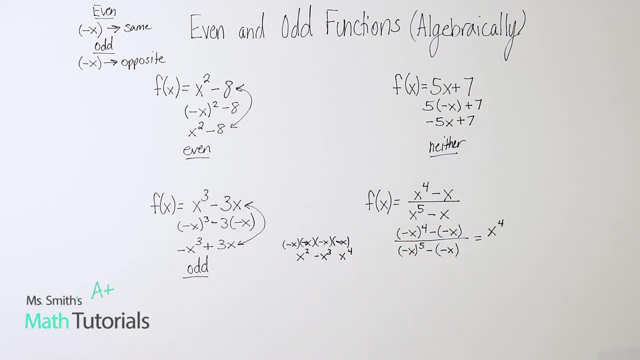 don't have to walk through this every time. but if that helps you, if it's positive, it's just if it, excuse me. if it's even, it's going to come out to the positive version, all right. and then negative times: a negative, that's a negative. 1 times a negative, x, which would be a positive x. 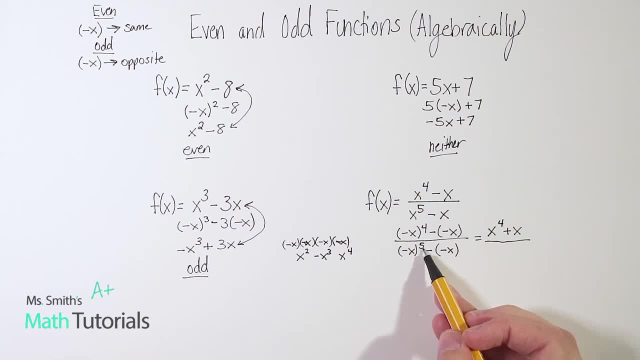 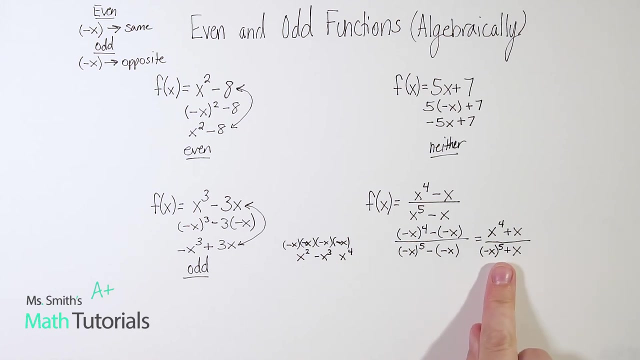 let's reduce the bottom. so: negative x to the fifth. we could write it out kind of like this, or we could just recognize that's an odd number. so this is going to end up being a negative x to the fifth. it's going to stay negative and then negative 1 times. negative x is positive x. okay, now let's compare that to. 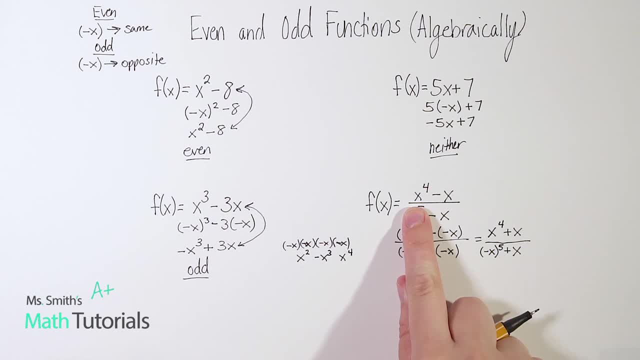 what we had to start with. all right, the x to the fourth was positive. it's still positive. this was a negative x, this is positive. so right here i can say: all right. well, we definitely are not the same. we're not the exact opposites. this is neither. 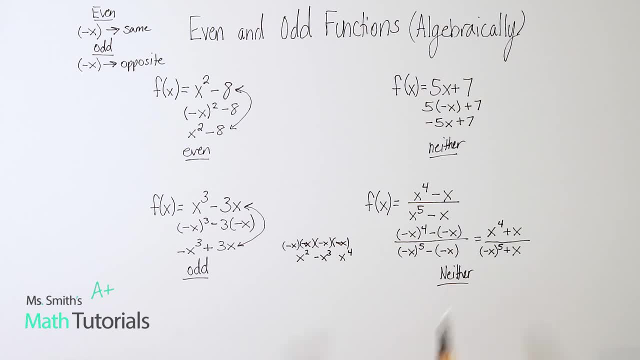 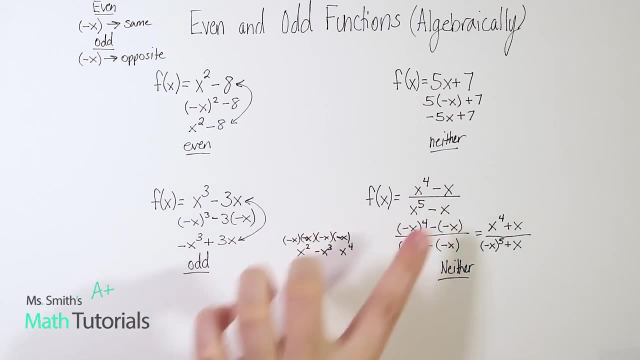 i could double check the bottom just to confirm, but you'll find the same thing. it's, they're not. they're not the same or opposites, and let me just confirm. let's see how this looks on the calculator. now this looks a little weird. you may be thinking: how are we going to put that? 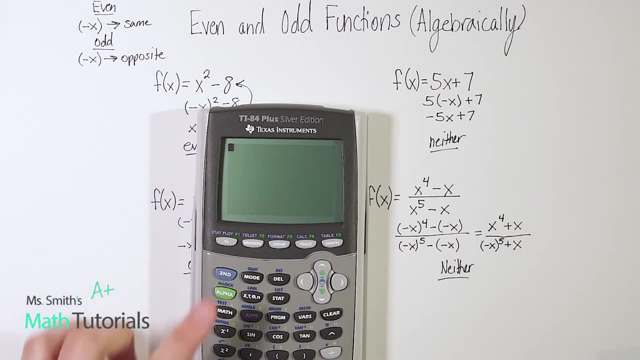 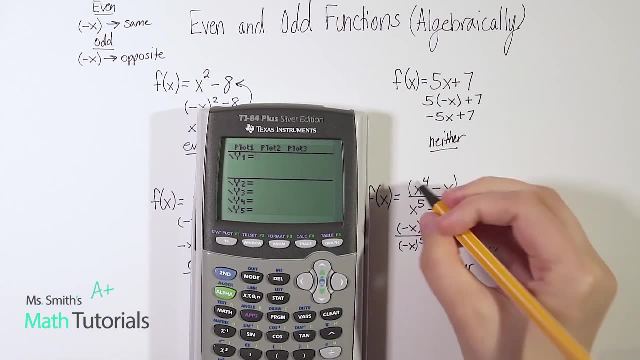 in for y equals. we're going to use our parentheses, so we would go to our y equals. we want to do a parentheses over everything up top and a parenthesis over everything in the bottom. so now i'm going to input. we're going to put this one totally in. x to the fourth. 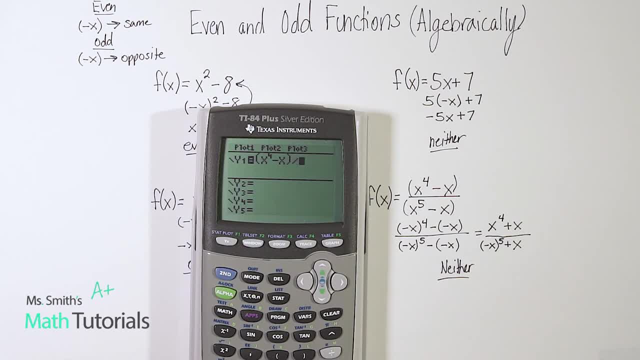 minus x, close that parenthesis out. divided by open another parenthesis, x to the fifth, minus x, close that parenthesis out. and let's look at it. yeah, so if i look at the y- yx, it's definitely not, even, it's definitely not perfectly reflected or mirrored. and then if i were to flip this upside down, note those characteristics. so at the bottom we got kind. 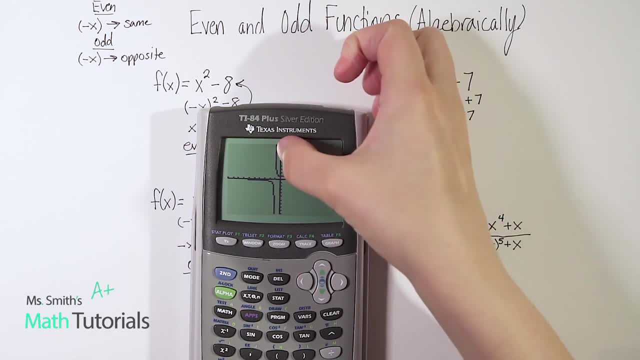 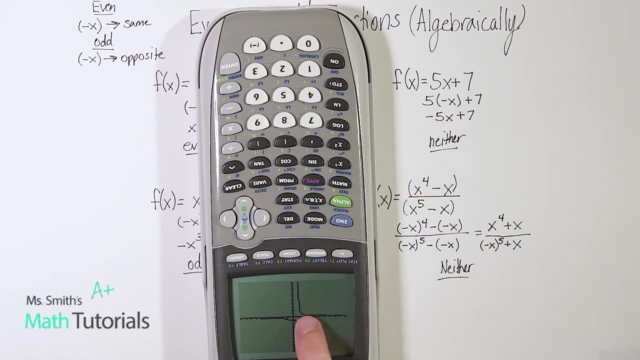 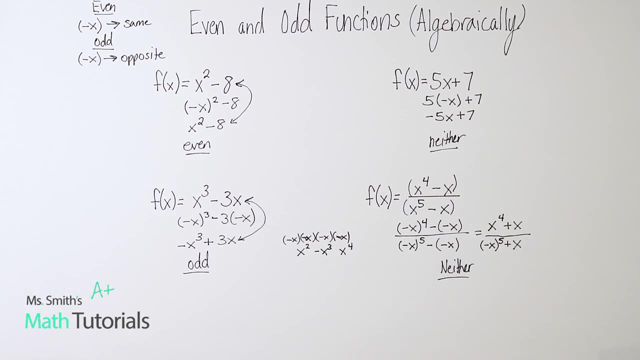 of a strip of space here and a smaller strip of space up here. if i were to flip it now, my strip of space is over on the right side. it was on the left, so, looking at this, definitely not odd. or even so, it's going to be neither. 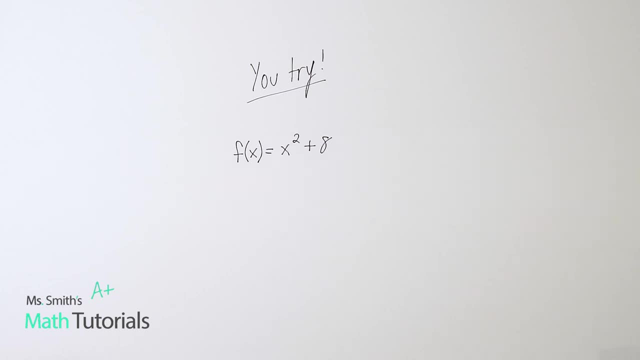 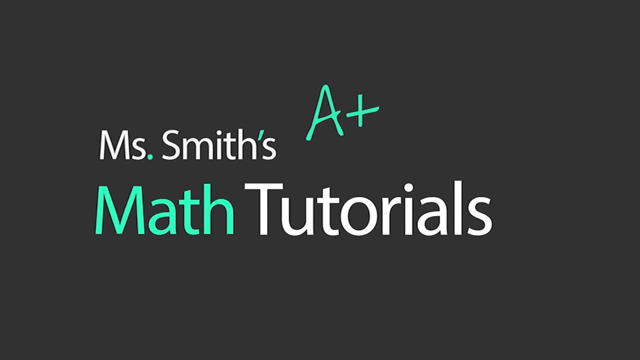 so you guys, try this one, determine if it's going to be even odd or neither. the answer you'll find in the description of this video. this has been miss, miss math tutorials.